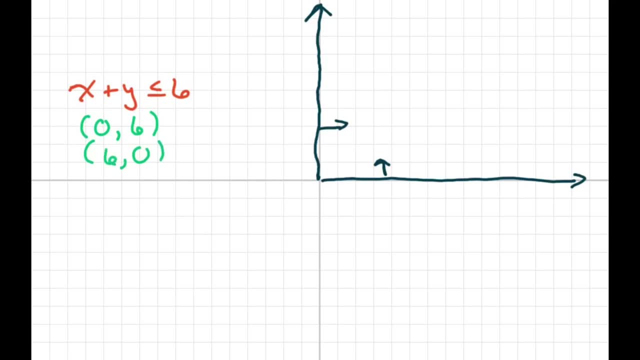 So that's a six. So we'll do that in red. I'm going to go up to six: One, two, three, four, five, six, And then we have one, two, three, four, five, six, All right. 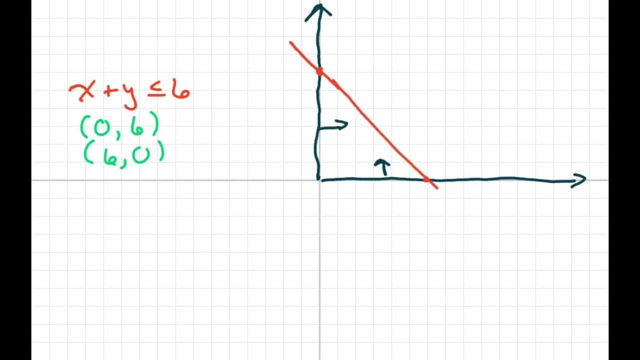 Oh, let's see. Oh, that's as best as I'm going to get, All right. So, anyway, this means all values are equal. So we're going to go ahead and get started. So we're going to go ahead and use less than six. If I plug in zero, zero, that works because zero plus zero. 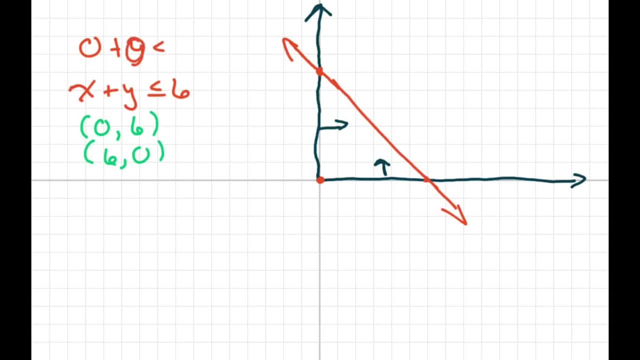 is indeed less than or equal to six. This would be a zero, So I know it's going to be shading down Anytime. it says less than it's either down or to the left. So we're in this area, And the other constraint we have is x plus y is greater than or equal to one, And 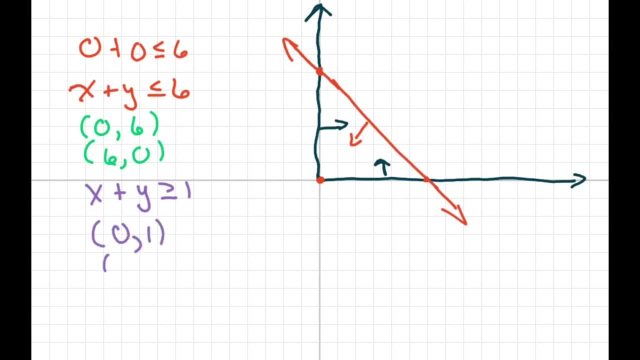 for if x is zero, then y is one, And when y is zero, x is going to be one. So we're right in here And kind of graph that. So that means we're shading in this area here, because that means it's greater than That means we're shading up, So you can just shade, do a crosshatch. 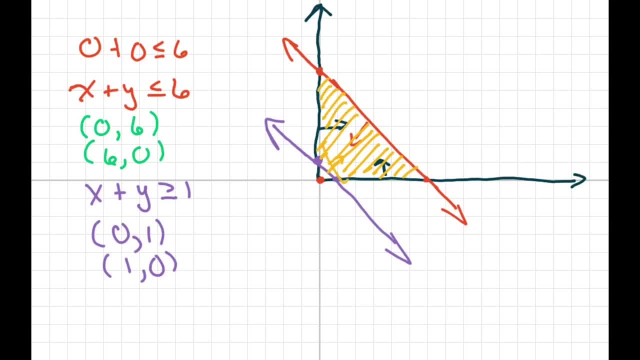 type thing here, or just shade in there, Color it all in. But that's our area. So I'm going to go ahead and write my corner points. This one right here was zero comma six. This one here is zero comma one. This: 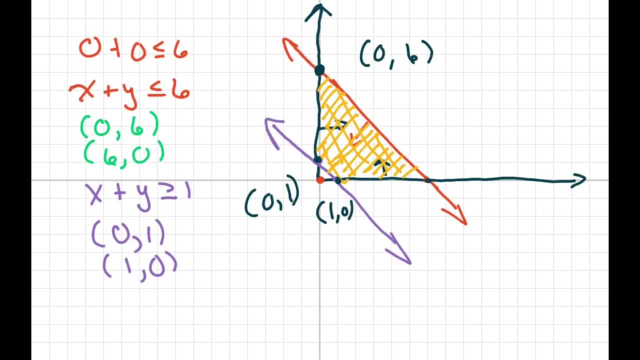 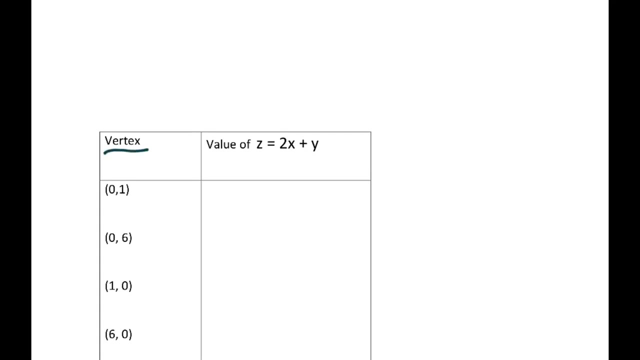 is one comma zero And this is one six comma zero. So those are your corner points that we're going to use to maximize our equation. So I went ahead and took the liberty of writing them And I'm going to write them down. Those are vertex points, And we merely just plug them. 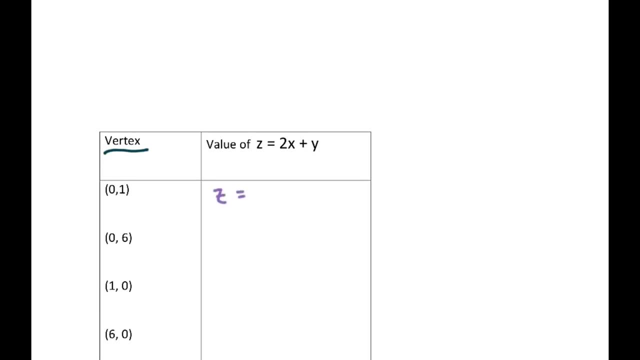 in. So we have z equals two times zero plus one, which equals one. For this one, we have z equals two times zero plus six, which equals six. For this one, we have two times one plus zero, which equals two.